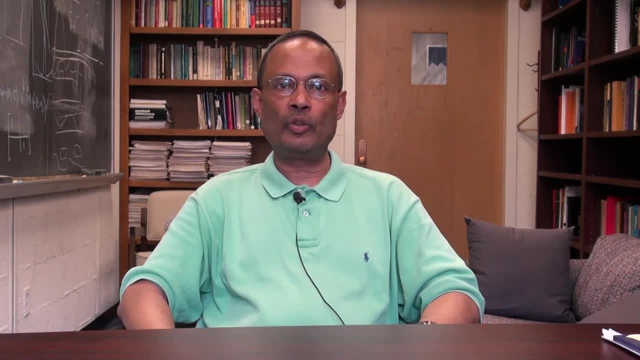 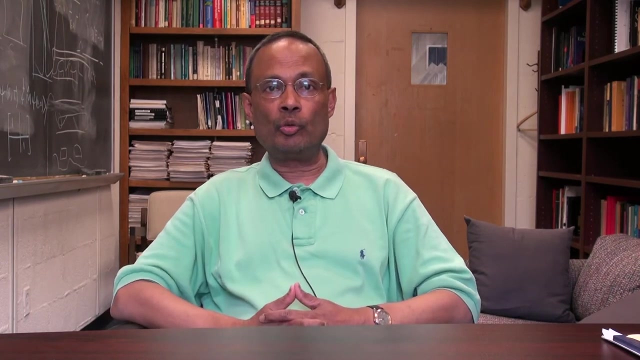 Hello, I'm Shankar Das Sharma of the University of Maryland, and today I'll be talking about fractional quantum Hall effect, which is one of the most amazing and also one of the most important physics discoveries of the last 50 years. What was discovered by Suey Stormer? 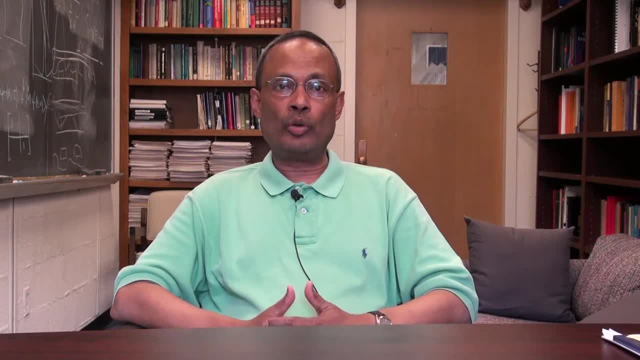 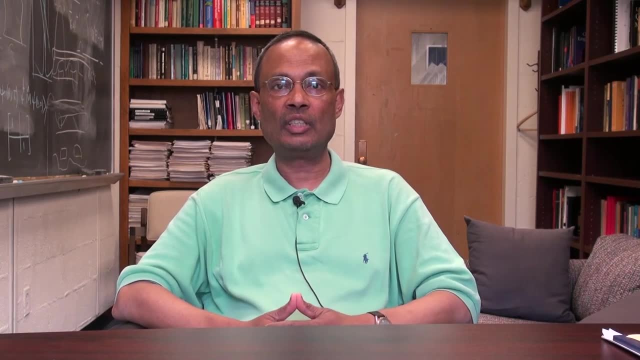 and Gossard of Bell Laboratories in 1982 was: when you go to a very high magnetic field, a two-dimensional electron gas happens to be semiconductor. that's why they exist. shows fractional quantization of Hall conductance in units of E square over H. Now what do I? 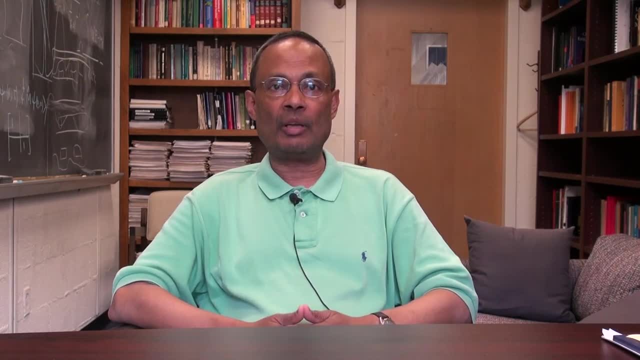 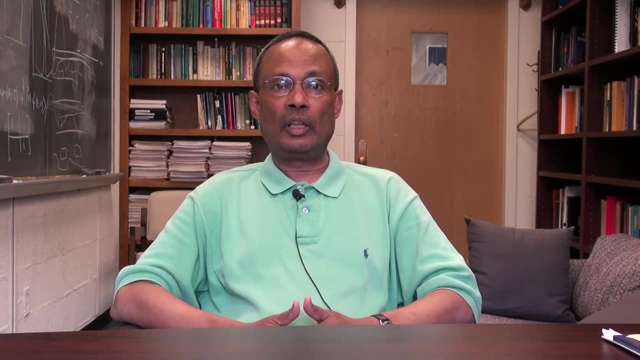 mean by fractional quantization. Well, let's take a step back and talk about integer quantum Hall effect a little bit. In 1980,, Claus von Glitzing discovered that a two-dimensional electron gas subjected to a very strong magnetic field shows integer quantization, which basically: 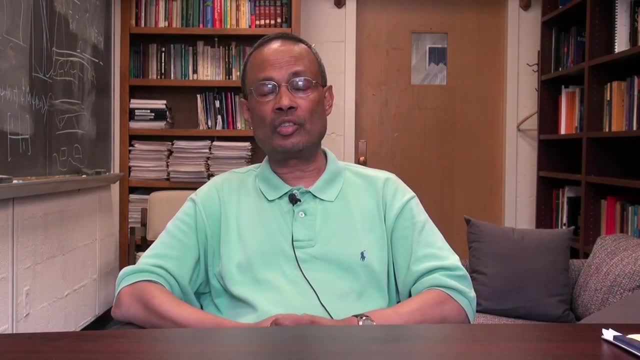 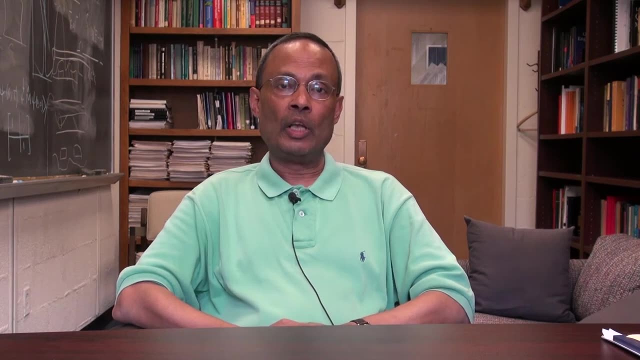 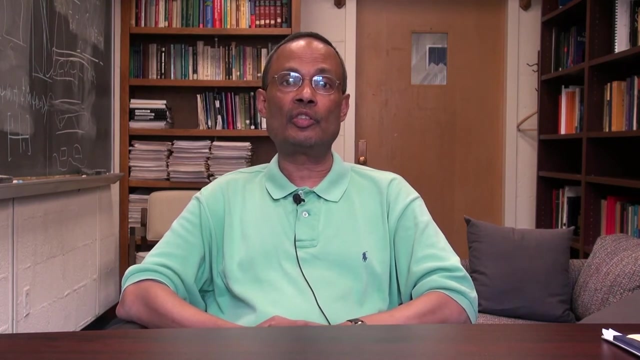 means that the Hall resistance, Hall conductance, is quantized in units of E square over H, when you have an integer number of Landau levels occupied. When you apply a strong magnetic field to a two-dimensional electron gas, the system decomposes, the density of cells decomposes. 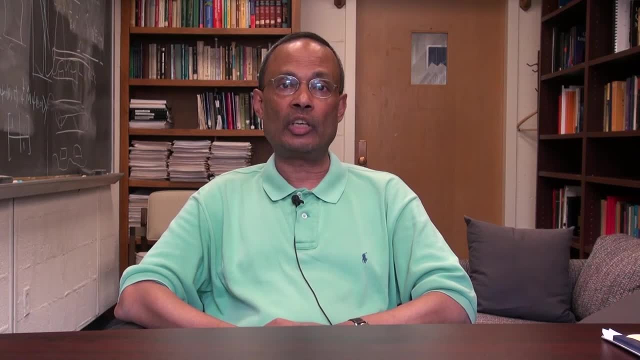 into a bunch of Landau levels. So as you move the chemical potential or as you increase magnetic field, that means as you change electron density or you change magnetic field, your Fermi level is going to change, And that's what we're going to talk about in the next. 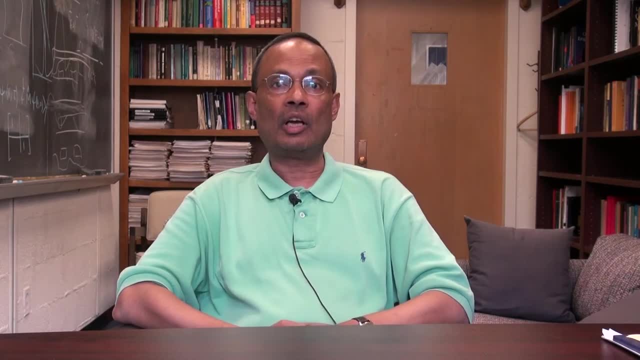 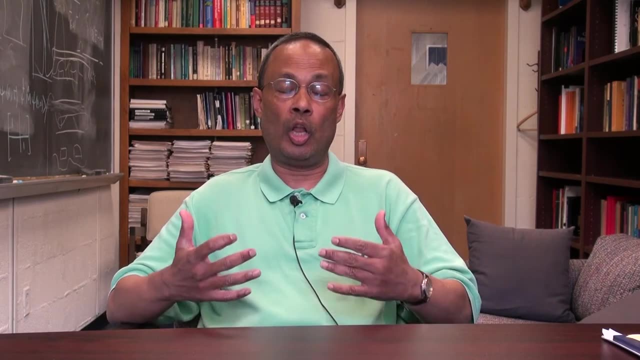 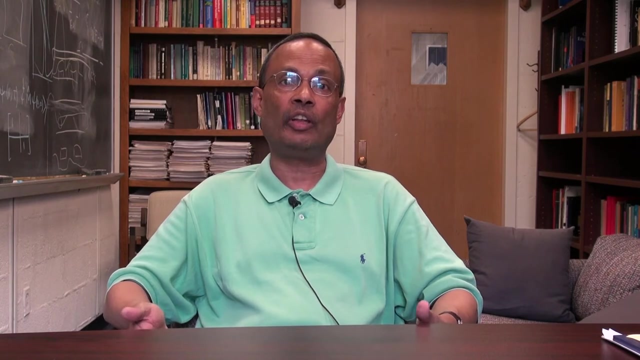 lecture, So you can have a certain number of Landau levels occupied. And what Claus von Glitzing found? that the quantum, the Hall resistance or Hall conductance is quantized, and the quantization number corresponds to the number of integral filling of Landau levels. So it was natural. 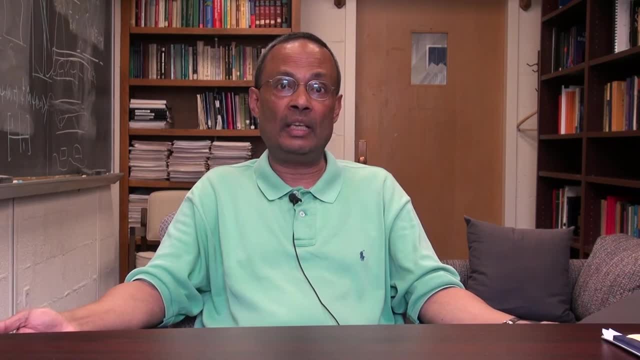 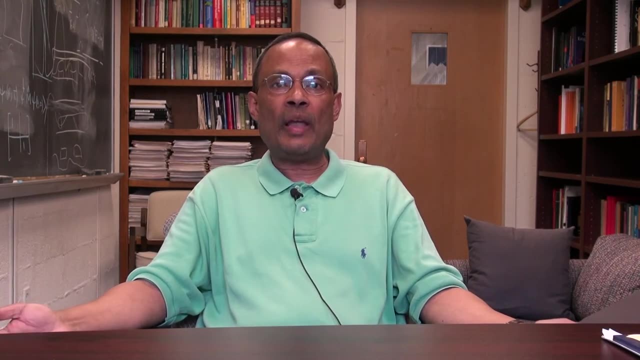 to go to a situation where the lowest Landau level is occupied, meaning make the magnetic field large enough so that you have partial filling of the lowest Landau level- What we expected- and I was an active researcher at that time, so I remember the feeling precisely. 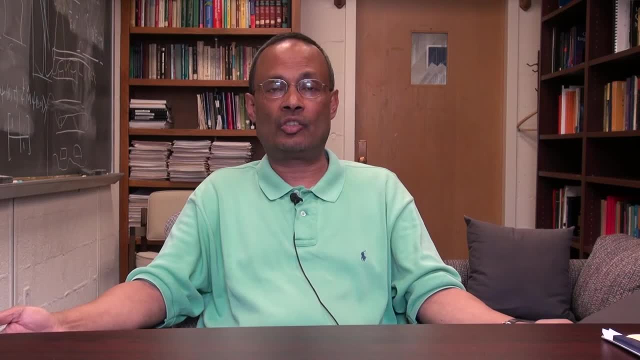 We all expected that the system will form some kind of lattice called Wigner crystal or perhaps a charge density wave. Why? Because you know the system would want to minimize potential energy. When you go to the lowest Landau level, you basically have no kinetic. 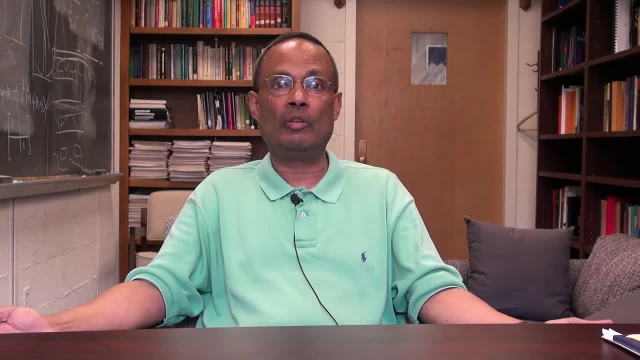 energy left, Right, You have only zero point energy. H bar omega C divided by two It's a constant. See, if all the Landau levels are well separated, that means in the high magnetic field limit you just have to have a well separated amount of energy. So the energy 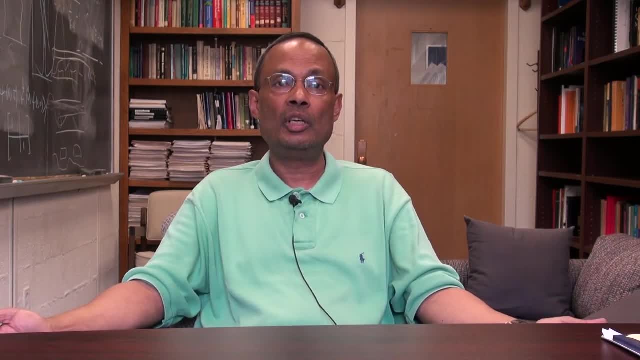 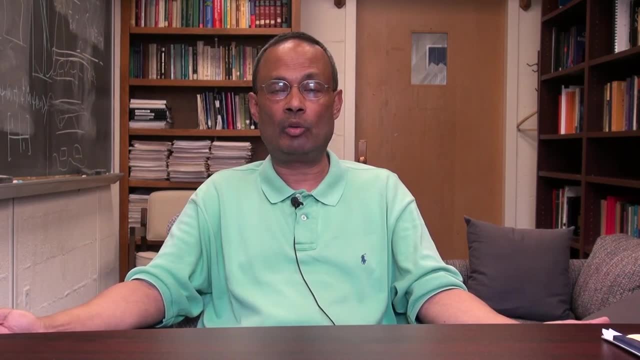 of potential energy. Well, we thought the system will minimize potential energy by forming a lattice. just as ions form in a solid, Ions form a lattice, electrons form a gas or a liquid. The reason is that ions are trying to minimize potential energy and, in a quantum system, minimize potential energy. 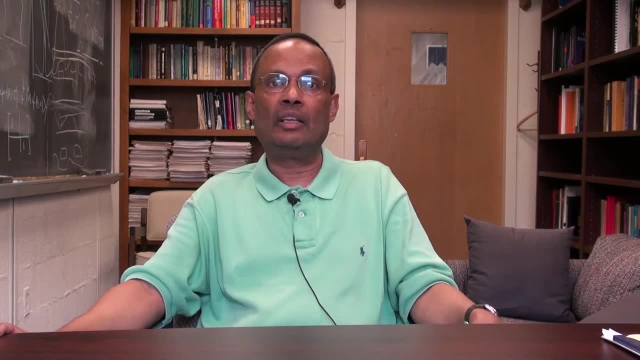 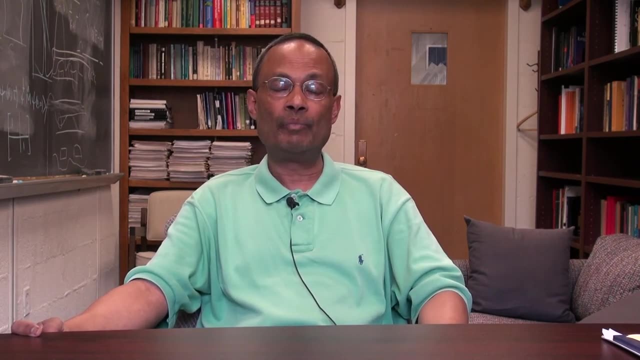 by staying away from each other, by forming a lattice. Well, that didn't happen. What happened, we found out, is the system formed an incompressible quantum liquid. Bob Laughlin wrote down a wave function for this liquid and it showed that you have gaps. 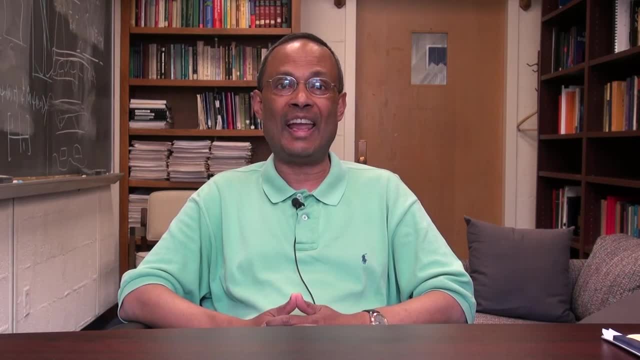 at this fractional filling, where the fractional filling goes as one over m, m being an odd denominator. So the original fractional fraction one-third. now we know it can happen at one-fifth and so on. But later on we found out that this fractional quantum Hall effect can take place. 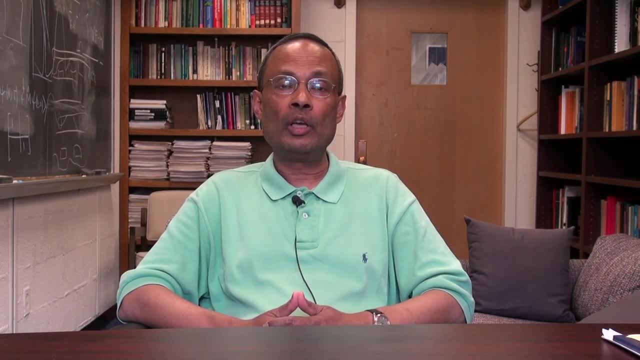 generically at any fractional filling p over q, where q is an odd number and p could be anything. Why The reason? The reason is the system actually minimizes energy by forming an incompressible quantum liquid, by forming gaps at these odd denominator fractions. 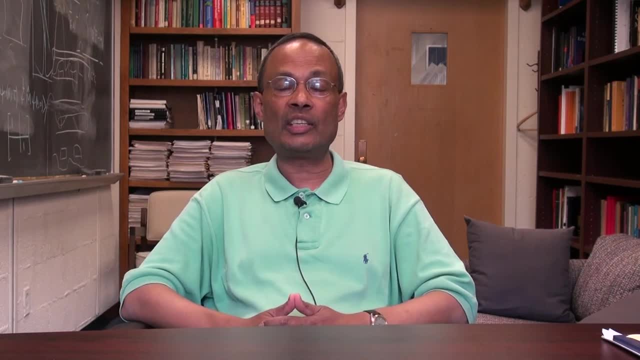 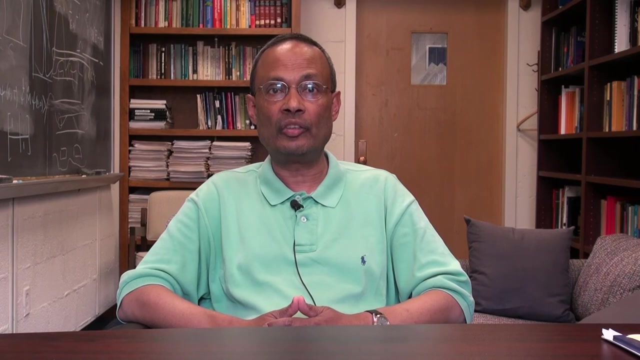 Very strange system where the minimization is associated with the formation of an incompressible quantum liquid. And it's incompressible because there is an energy gap. Now we know from integer quantum Hall effect that having a gap is equivalent to having quantization of the Hall resistance or Hall conductance. 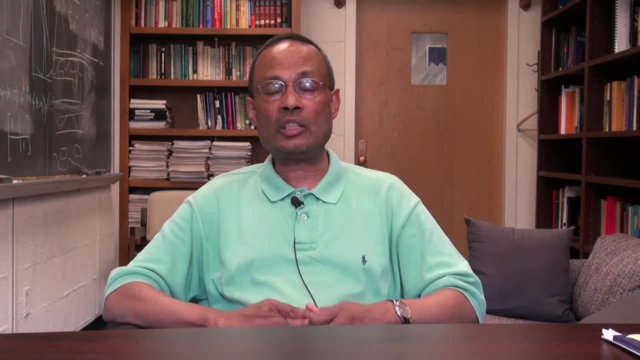 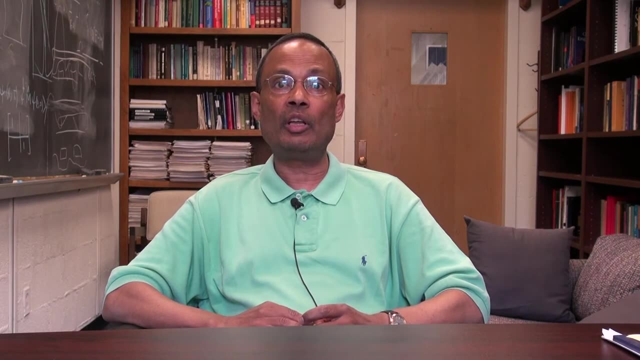 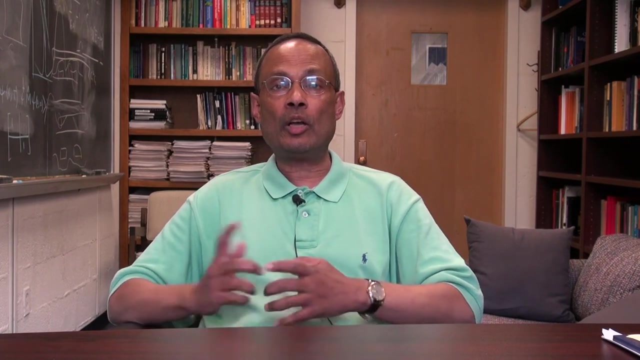 So that's exactly what happens in a fractional quantum Hall effect, Just like integer quantum Hall effect, the Hall conductance is quantized, but now not at integer filling, but at fractional filling, because the system has formed this incompressible, strongly correlated liquid, because the original non-interacting system had a macroscopic degeneracy. 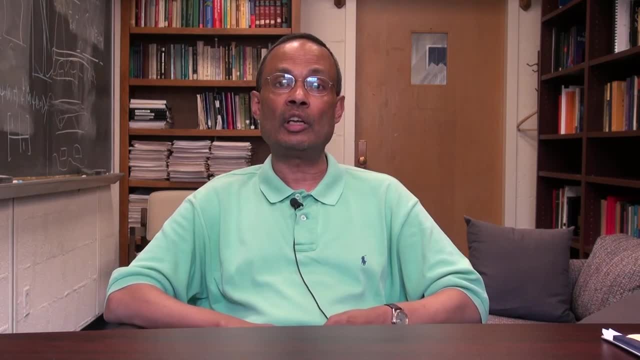 All the electrons in the thermodynamic limit, infinite number of electrons. but even for real system, trillions of electrons, billions of electrons have increased in number, Exactly the same non-interacting energy. So the system has this macroscopic degeneracy which leads to this very strange, incompressible liquid.